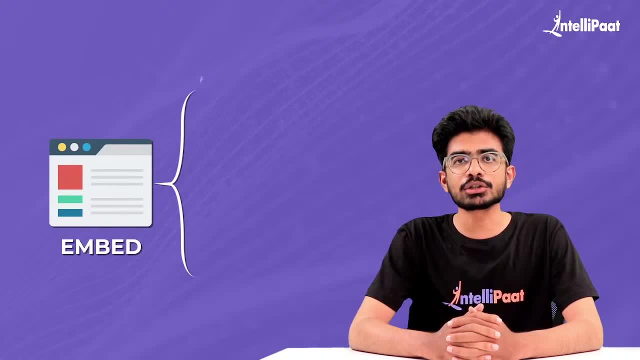 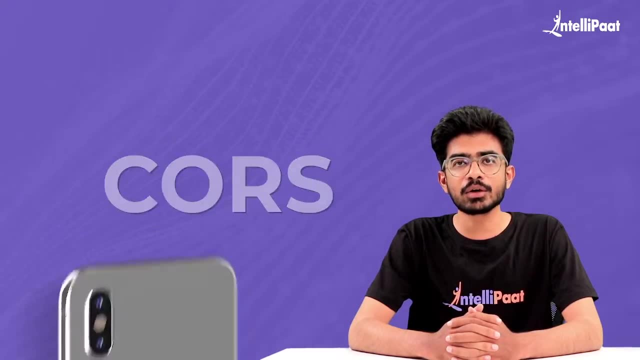 resource loading. A web page freely embeds cross-origin images, style sheets, scripts, iframes and videos. Let us learn more about CORS in this video, but before that, make sure that you subscribe to our YouTube channel and hit the bell icon for regular updates. 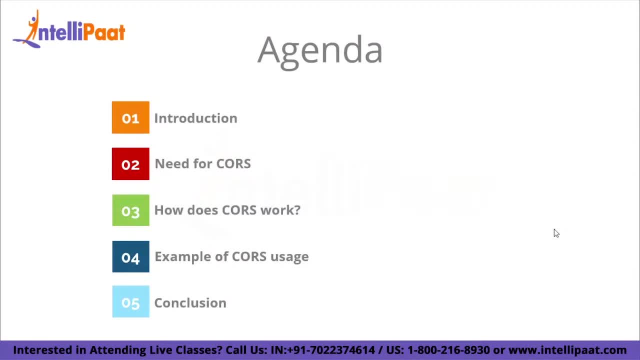 All right, now let us take a look at the agenda for this video. Firstly, I will be introducing the concept of CORS. Next, I'll move on to the need for CORS, the reason why CORS came into existence. It is basically a mechanism. 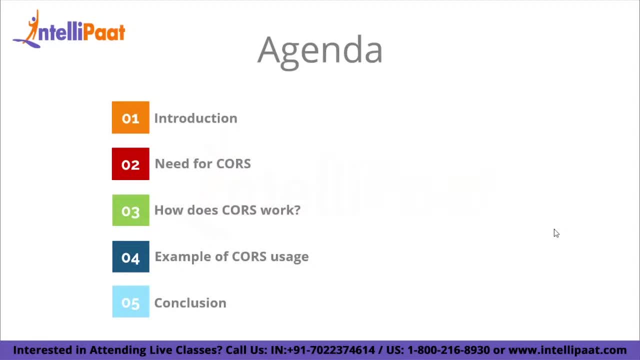 And next I'll move on to the topic: how does CORS work? We have four steps in how CORS works. I'll be explaining each one of them in this section and later I'll be taking up an example of the use case of CORS. 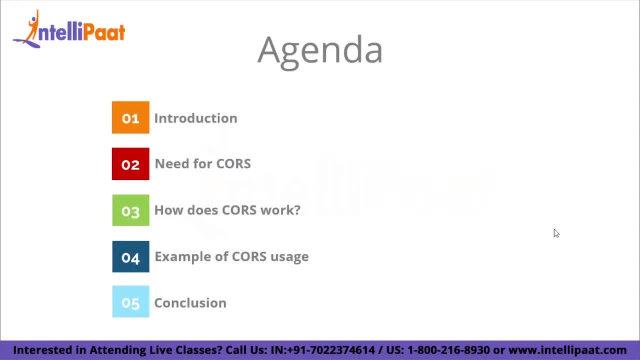 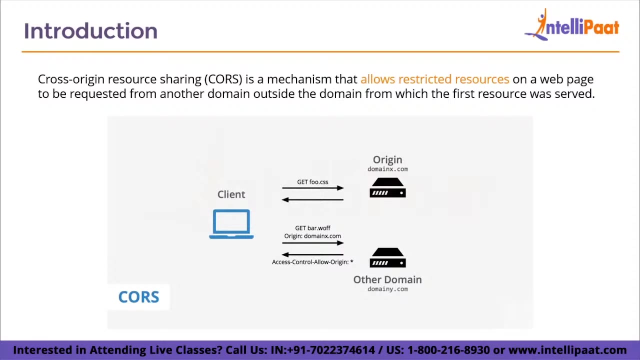 That is where it is used in the real world. And finally, we'll be taking a look at the conclusion of this video. Now that we are clear with the agenda, let us move on to the first topic: introduction- Cross-origin resource sharing, which is an acronym for CORS. 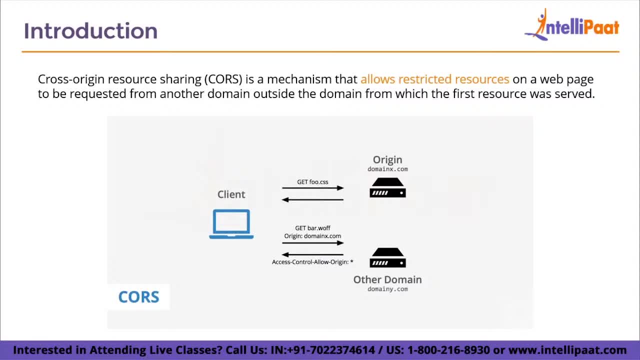 It is a mechanism that allows restricted resources on the web page to be requested from another domain outside the domain from which the first resource was served. So in simple terms, let's say a client from a web browser makes a request to a domain. 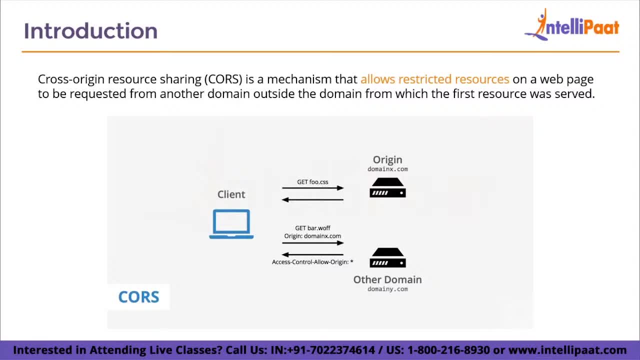 that is basically a server And this first domain is called as domainxcom. And let's say, we have another domain called domainycom And the web page you are requesting has some image which is not present in domainxcom. It is actually present in domainycom. 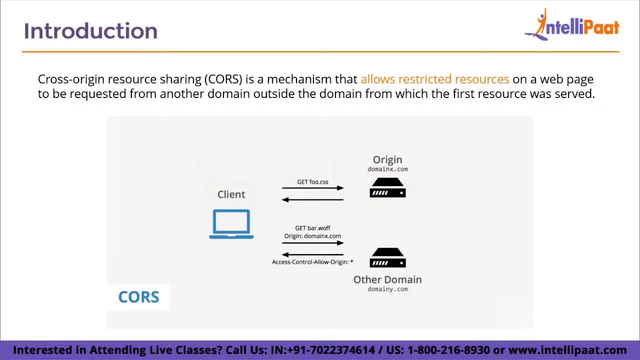 So how do you get this? How do you get this image? So you make a request to domainxcom and in turn it gives you the web page, but without the image, because the image is present in domainycom. And then you make a request again to another domain, which is domainycom. 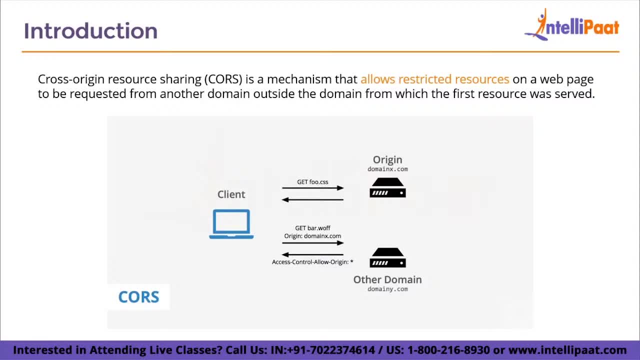 And if that clears, if the security checks are clear, then you will be allowed access to the image file that is present in the domainycom And basically, after all these steps- that is all the four steps- you will get the web page as well as the image embedded on it. 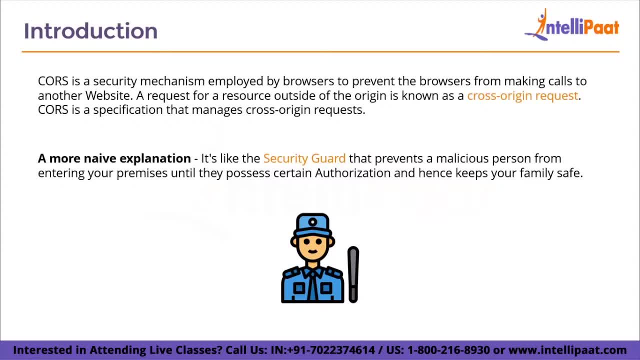 Now let us see an alternative definition. In other words, CORS is a security mechanism employed by browsers like, let's say, Firefox, Chrome, Internet Explorer, etc. to prevent the browsers from making calls to another website, A request for a resource like an image or a font, etc. 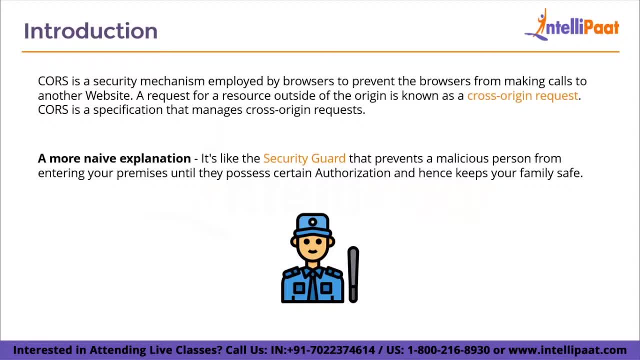 Outside of the origin is known as a cross origin request. CORS is specification. It is basically a specification that manages cross origin requests. Now let us take a look at the base level explanation. that is a naive explanation for it. It is like the security guard that prevents a malicious person from entering your premises. 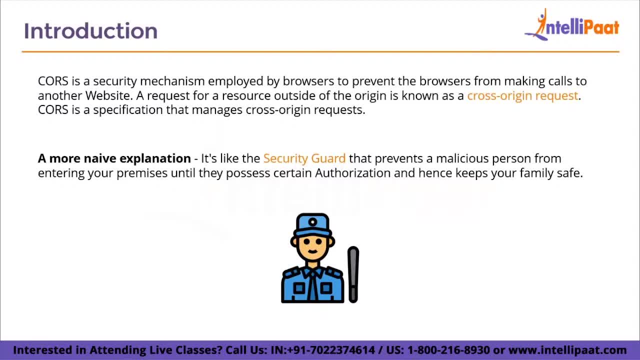 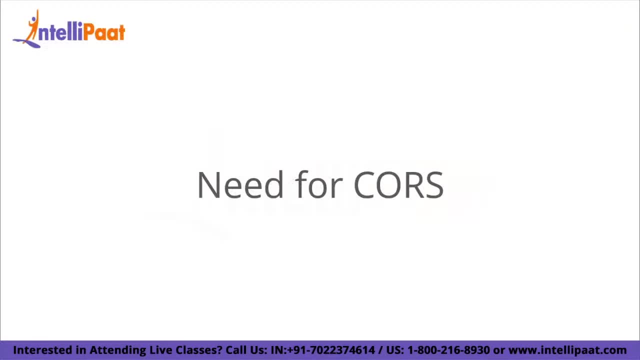 until they process certain authorization or an ID card, Let's say- and hence keeps your family safe. I hope that by this time, you guys would have had some rough idea of what CORS is. Now, to make things more clear, let us move on to the next topic, which is need for CORS. 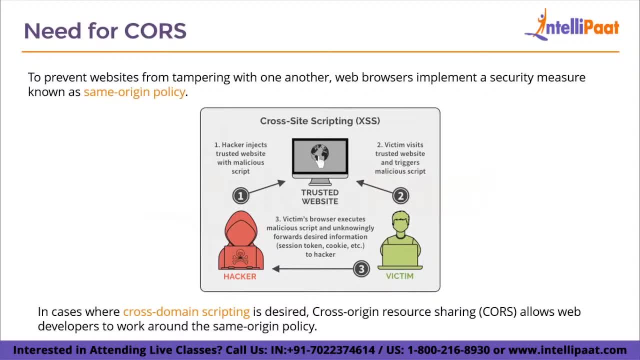 To prevent websites from tampering with one another, web browsers implement a security measure known as same origin policy. Now, what is the same origin policy? This policy lets resources such as JavaScript interact with other resources from the same domain, but not with resources from different domains. 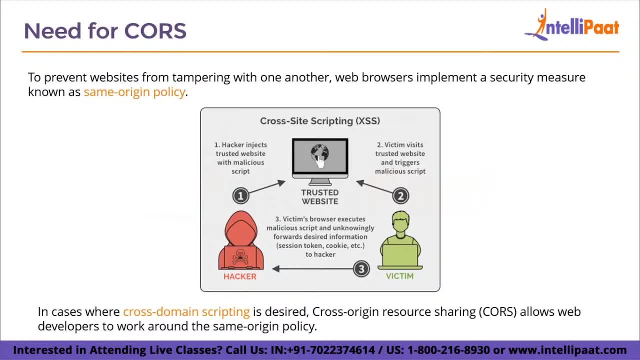 So this is, by default, the security measures. by default is that resources like JavaScript can interact with resources from the same domain and not with different domains. This provides security for the user by preventing abuse, such as running a script That reads the password field on the secure website. 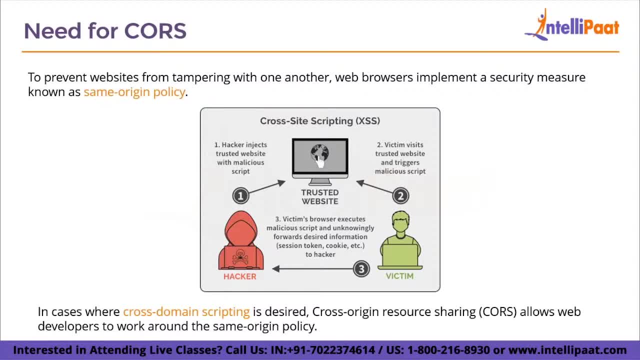 So, basically, this security measure is taken to avoid cross site scripting, or XSS, In cases where cross domain scripting is desired. cross origin resource sharing, or CORS, allows web developers to work around the same origin policy. CORS adds HTTP headers that instruct web browsers on how to use and manage cross domain content. 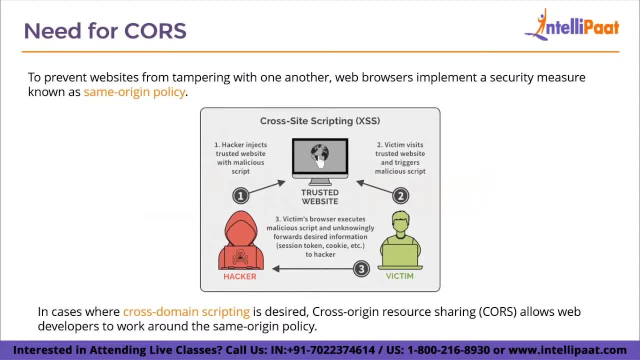 The first thing that you need to know about CORS is that you need to know how to use and manage cross domain content. The browser then allows or denies access to the content based on its security configuration. That is, if the HTTP header has the CORS content, it is allowed inside the domain. 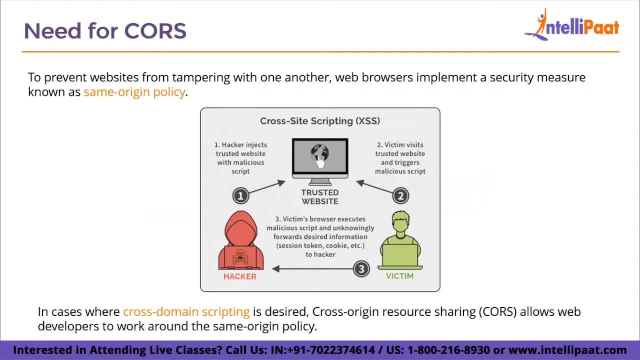 If not, it is not allowed. Just like the security card has his authentication or ID card with him, an HTTP header should have a CORS content attached to it, So if it has that, the domain will allow your CORS request. Now let us move on to how to use and manage cross domain content. 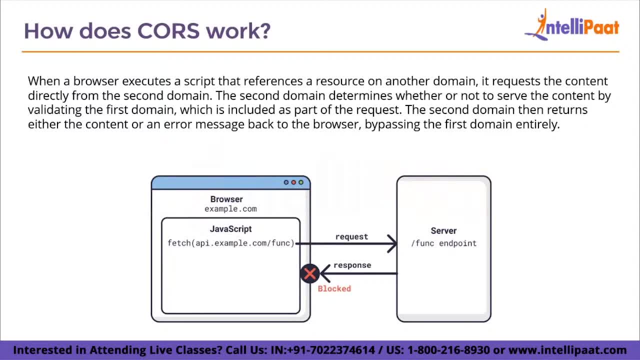 So how does CORS work? When a browser executes a script that refers a resource on another domain, it requests the content directly from the second domain. The second domain determines whether or not to serve the content by validating the first domain, which is included as part of the request. 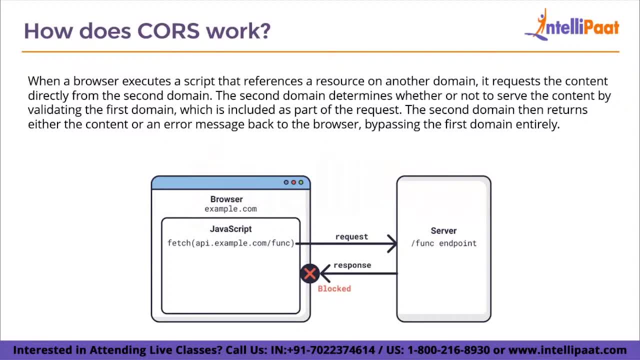 That is, the request coming into the second domain will already have the request of the first domain attached to it. The second domain then returns either the content or the source. The second domain then returns either the content or the source. The second domain then returns either the content or the source. 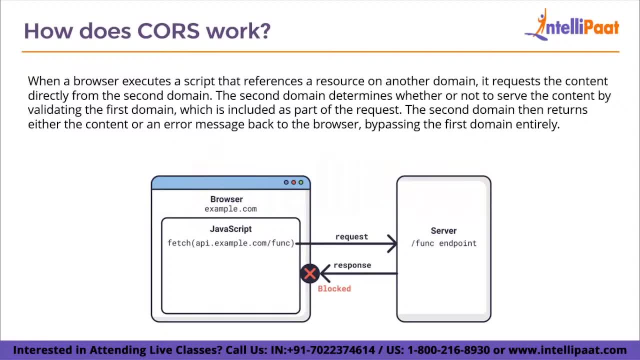 Returns either the content or an error message back to the browser, bypassing the first domain entirely, That is, After the second domain it acquires the request from the client. this request will obviously have the request from the first domain attached to it and it will see if the coarse security is correct or not. 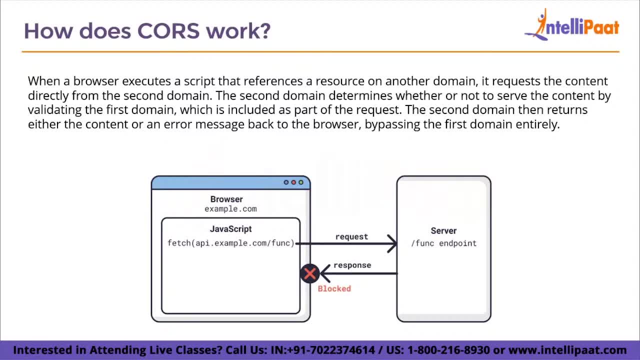 Jagj, If everything looks good on, if it needs to be구나, Everything looks good, it will serve the request bypassing the first server. or it will give you an error message, or it will be blocked, as shown in the figure. Now let us take a look at the step by step process of how course works. 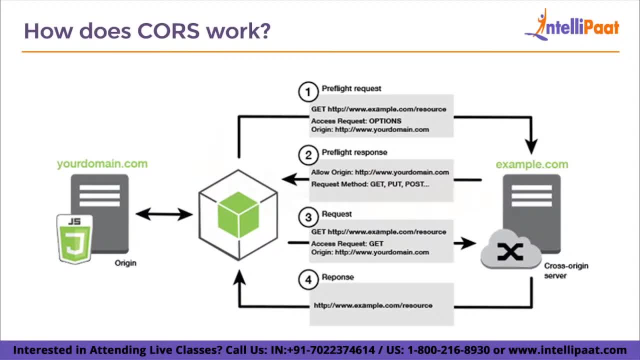 Step one: a user opens a resource on a page that references another domain. This is usually a javascript file, but can handle web fonts and css resources as well. And then the second step is the users browser creates a connection to the second domain, adding an origin http header to the request, which contains the first domain. 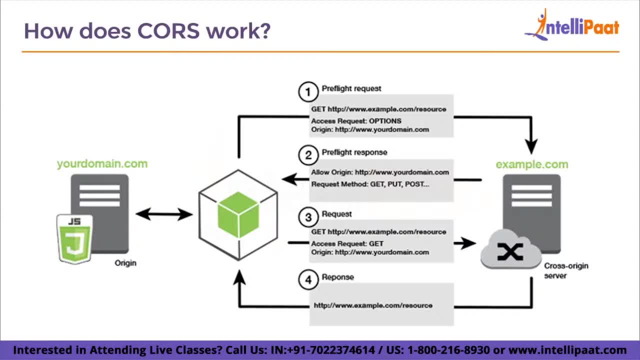 Now we will move on to the third step. The second domain replies with an access control origin http header which lists the domains allowed to make the call. Now the fourth step: if the first domain is allowed to make the request, the second domain responds with the requested content. 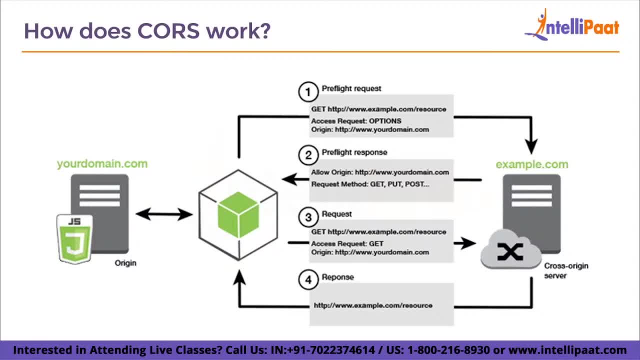 So this is how course works The access control allow origin header. now let us see what this means. It is defined in the second domain server configuration, that is, it will be present in the second domain. If the header doesn't contain wildcards and the first domain isn't explicitly included, the browser displays an. 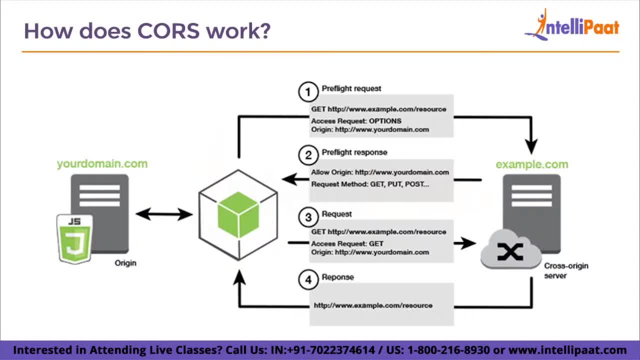 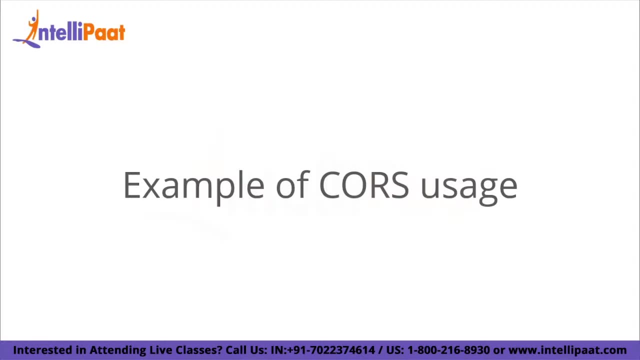 error message, That is, if the course header is not present in the request of the second domain, it will display an error message. So the first domain and the second domain should be configured properly for it to share resources. Now we will move on to an example of course usage. that is where it is used in the real 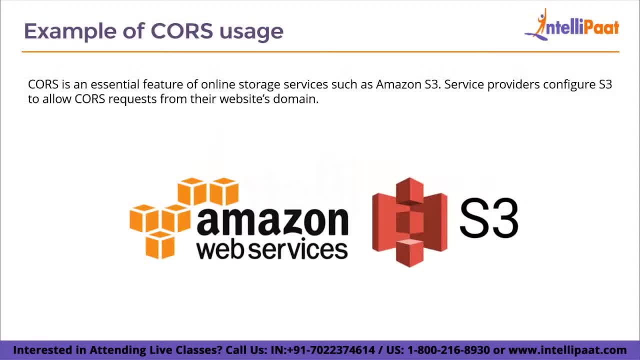 world. We will take one example. Course is an essential feature of online storage services such as Amazon S3.. So Amazon is a web service provider. It is the number one web service provider in the world right now and it provides a storage service called S3.. 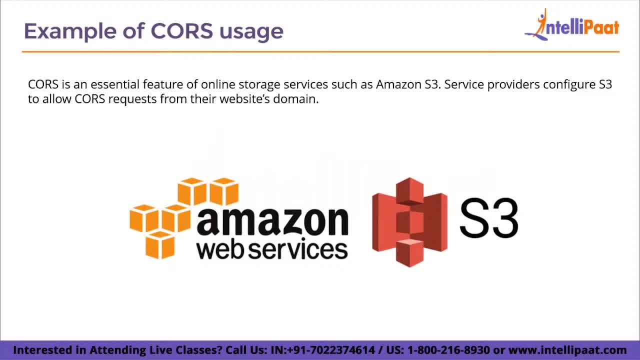 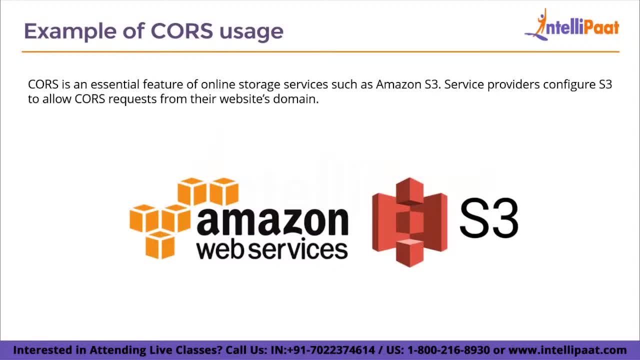 S3.. Since S3 is configured to allow the domain, That is, once you create the Amazon S3 buckets, you need to configure it to be able to accept course request And if that is done, everything goes well and the request is completed and the content is. 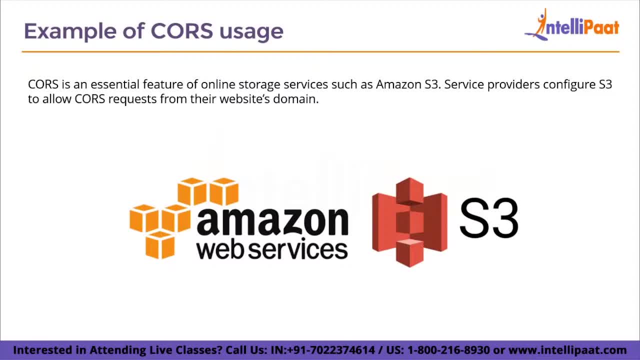 delivered to the browser Service providers, So Amazon S3 provides course capabilities as well in their S3 service. More complicated cross-domain requests use preflighting to validate a request before the request is actually performed. Preflighted requests include custom HTTP headers which help the server determine whether or